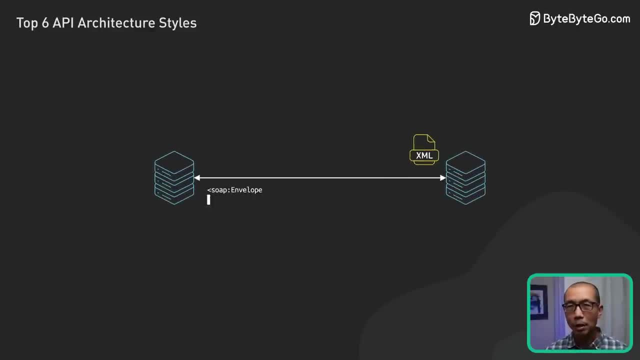 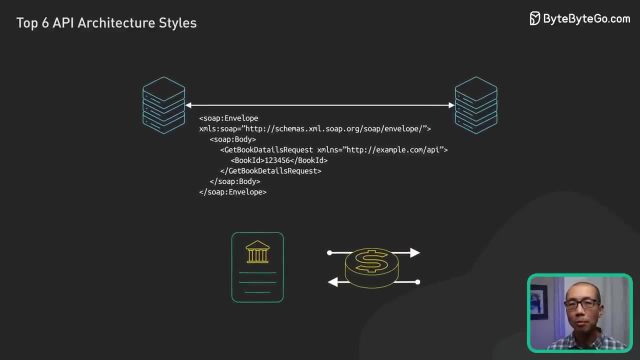 field. Mature, comprehensive and XML-based SOAP is heavily used in financial services and payment gateways, where security and reliability are key. However, if you're working on a lightweight mobile app or a quick prototype, SOAP might be overkill. It is complex and verbose. 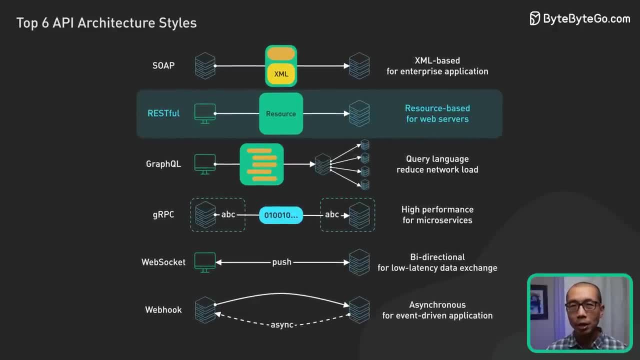 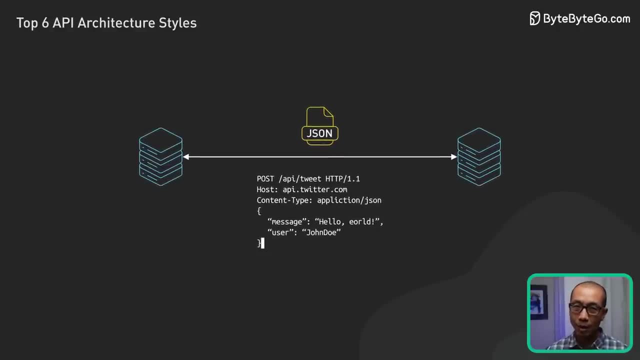 Then there's RESTful APIs. They are, like the internet backbone, popular and easy to implement. It's built on top of the HTTP methods. Most of the web services you interact with daily, like Twitter or YouTube, are powered by RESTful APIs, But if you need real-time data or operate, 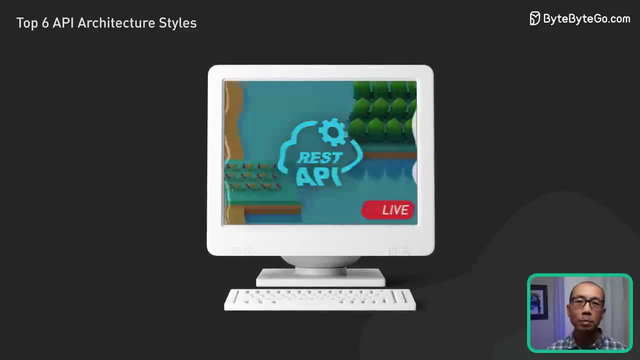 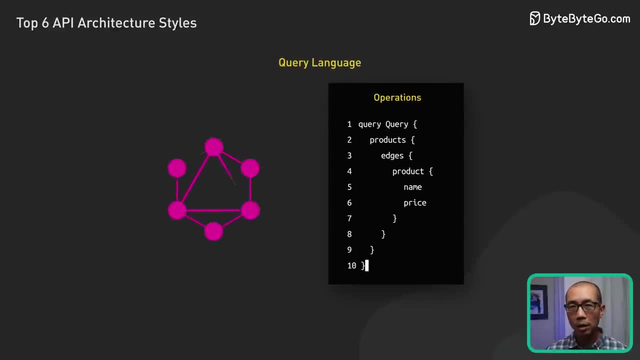 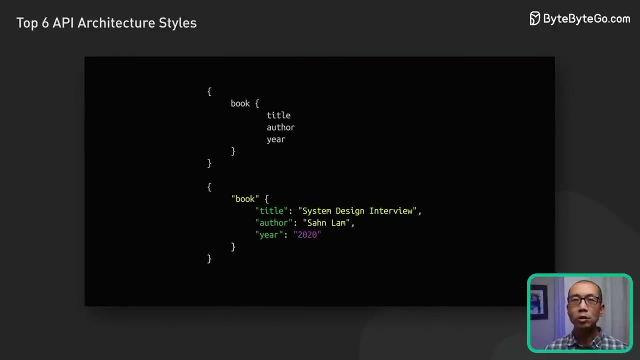 with a highly connected data model, REST might not be the best fit. Now let's turn our attention to GraphQL. It's not just an architectural style, but also a query language. It allows clients to ask for specific data as they need. This means no more overfetching or underfetching of data. You ask for exactly what you need. 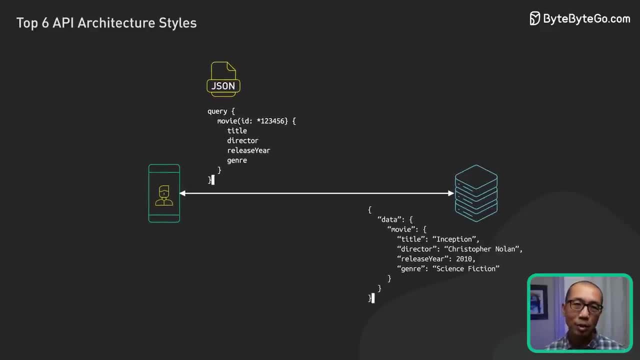 This leads to more efficient network communication and faster responses. Facebook developed GraphQL to deliver efficient and precise data to its billions of users. Now it is used by companies like GitHub and Shopify. Its flexibility and efficiency make it a strong choice for application with complex data requirements. 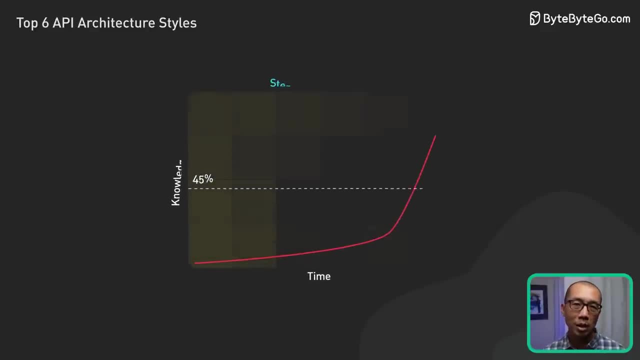 Now it's used by companies like GitHub and Shopify. Its flexibility and efficiency make it a strong choice for application with complex data requirements. But GraphQL does come with a steep learning curve. It also requires more processing on the server side due to its flexible querying capabilities. 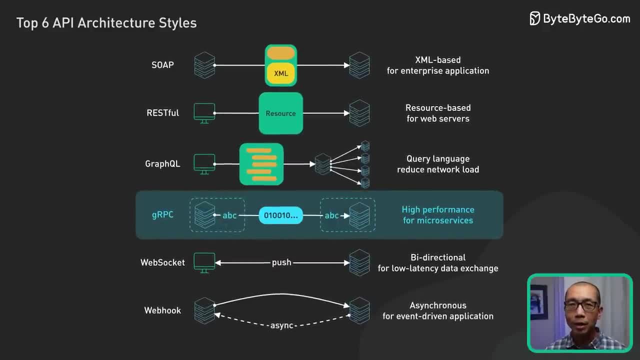 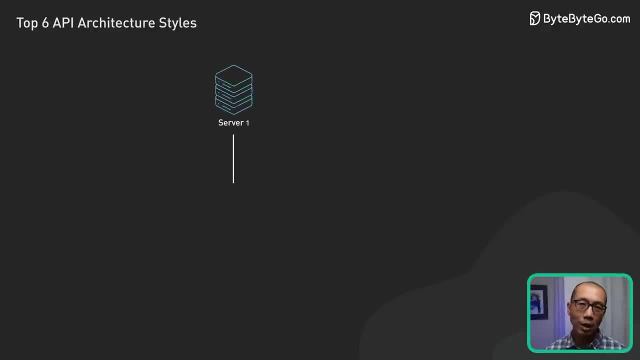 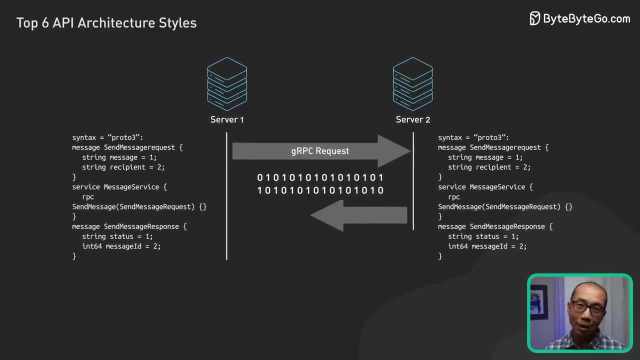 Let's talk about gRPC next. It's modern and high-performance. It uses protocol buffers by default. It's a favorite for microservices architectures, and companies like Netflix use gRPC to handle their inter-service communication. However, if you're dealing with browser clients, 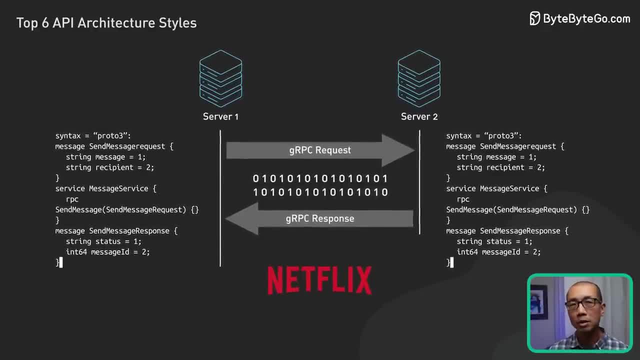 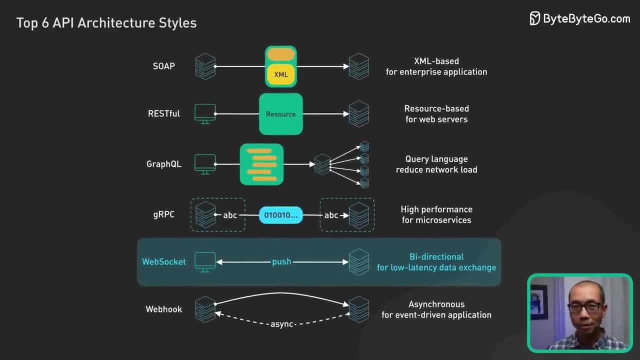 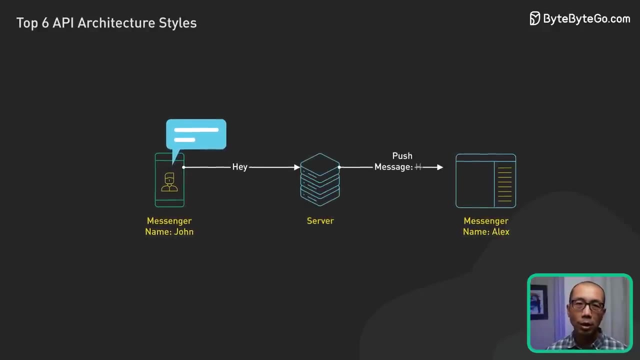 gRPC might pose some challenges due to limited browser support. WebSocket is all about real-time, bi-directional and persistent connections. It's perfect for live chat applications and real-time gaming, where a low-latency data exchange is crucial. But if your application doesn't require real-time data,